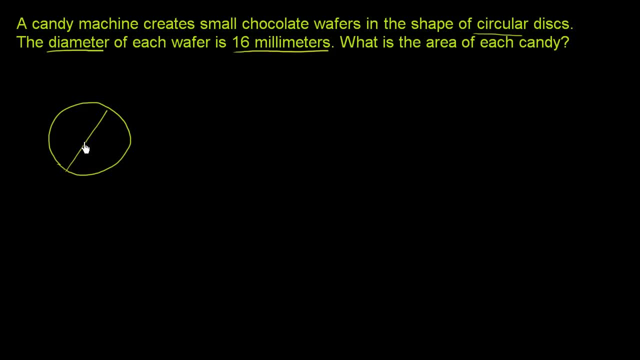 is 16 millimeters. If I draw a line across the circle that goes through the center, the length of that line all the way across the circle through the center is 16 millimeters. So let me write that. So diameter here is 16 millimeters. 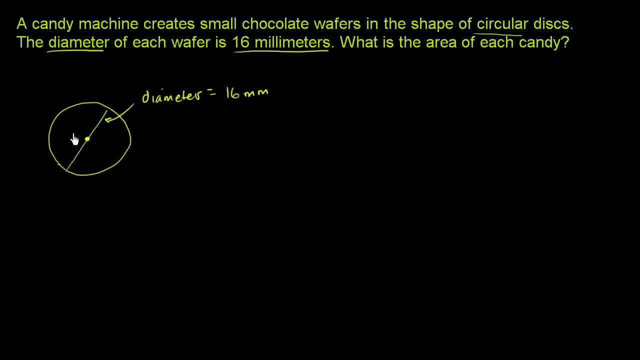 And they want us to figure out the area of the surface of this candy or, essentially, the area of this circle. And so, when we think about area, we know that the area of a circle is equal to pi times the radius of the circle squared. 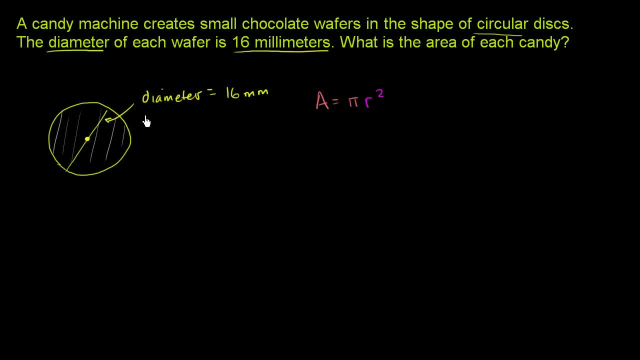 And you say: well, they gave us a diameter. What is the radius? Well, you might remember, the radius is half of diameter. It's the distance from the center of the circle to the outside, to the boundary of the circle. So it would be this distance right over here. 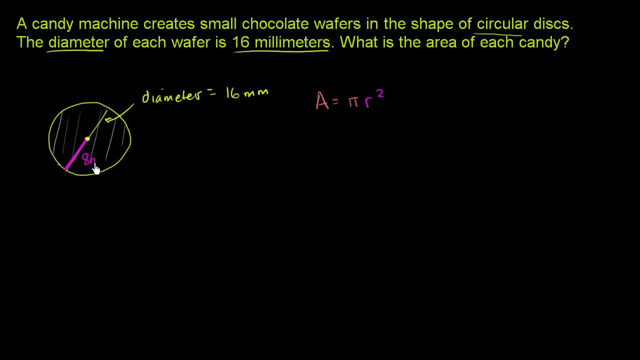 which is exactly half of the diameter, So it would be 8 millimeters. So where we see the radius, we could put 8 millimeters. So the area is going to be equal to pi times 8 millimeters squared, which would be 64.. 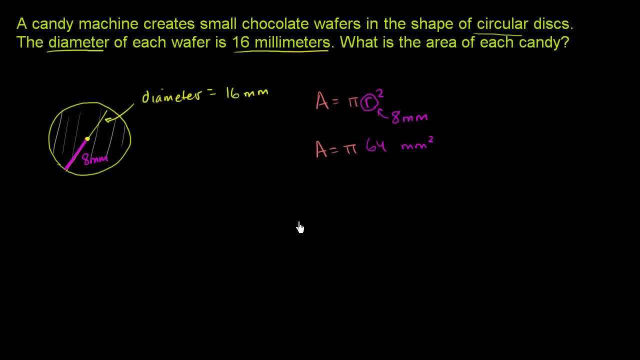 64 square millimeters, And typically this is written with pi after the 64. So you might often see it as this is equal to 64 pi millimeters squared. Now this is the answer: 64 pi millimeters squared. 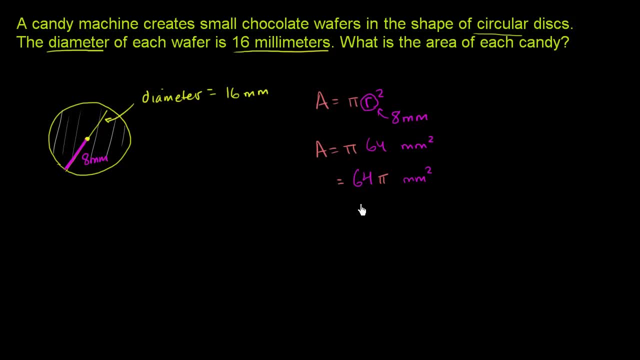 But sometimes it's not so satisfying to just leave it as pi. You might say: well, I want to get an estimate of what number this is close to. I want a decimal representation of this, And so we could start to use approximate values of pi. 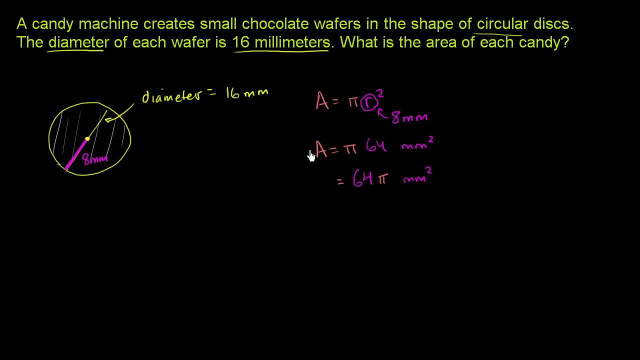 So the most rough approximate value that tends to be used is saying that pi- a very rough approximation- is equal to 3.14.. So in that case we could say that this is going to be equal to 64 times 3.14 millimeters squared.